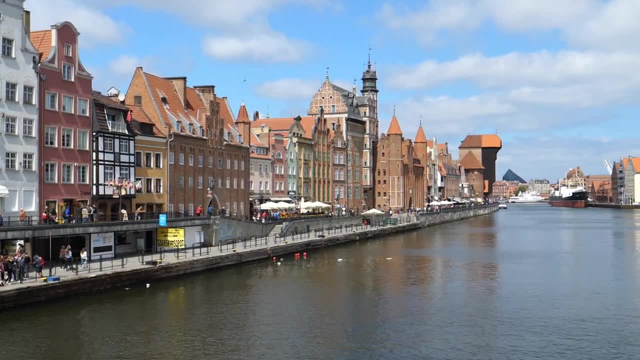 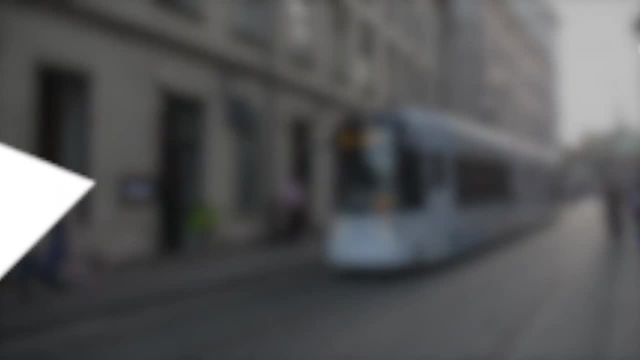 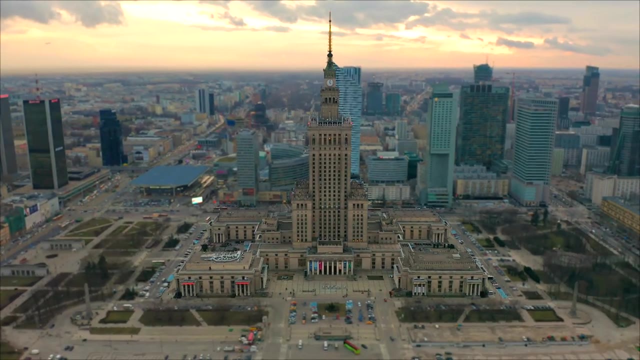 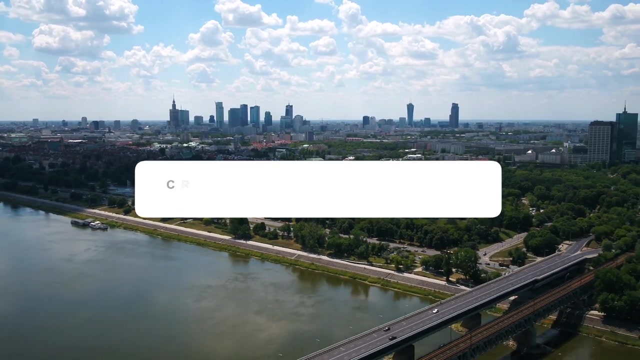 With a rich culture and interesting history, alongside vibrant cities and stunning scenery, there are many reasons to visit Poland. This is Katie from Creative Travel Guide, and today we look at how to visit Poland on a budget. Looking for more travel tips? Make sure to hit subscribe and ring that notification bell. 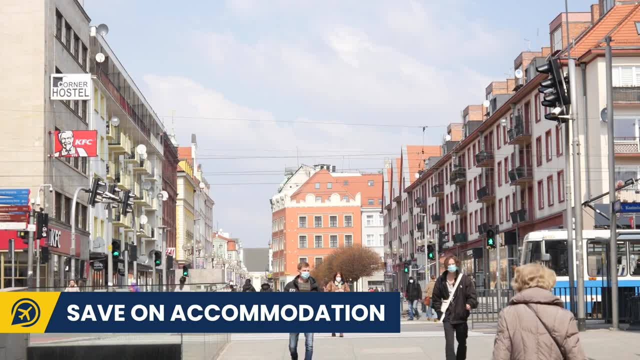 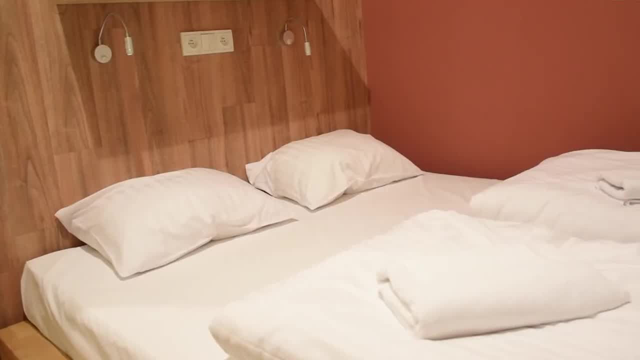 So, firstly, let's look at ways to save money on accommodation. There are plenty of hostels to choose from in Poland, with Krakow being home to some fantastic options. Dorm beds can be found from as little as $5 and are a great option for solar travellers. 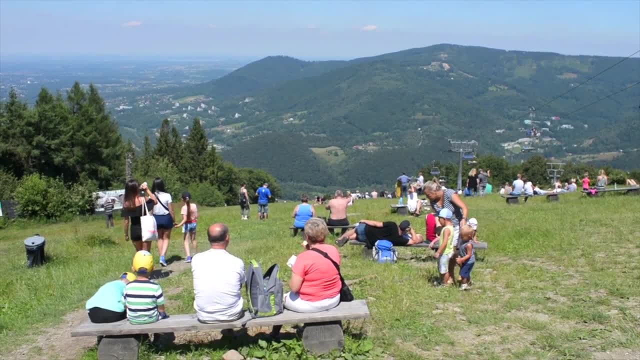 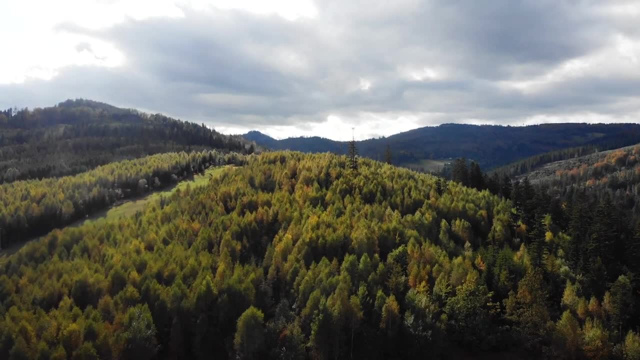 on a budget. If you are looking to stay in more rural areas of Poland, homestays and farmstays are inexpensive and a popular option in the country. If you are looking to book a hotel, avoid staying at a hotel in Poland. If you are looking to book a hotel, avoid. 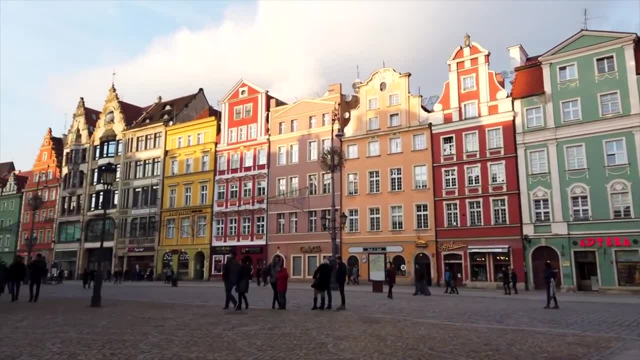 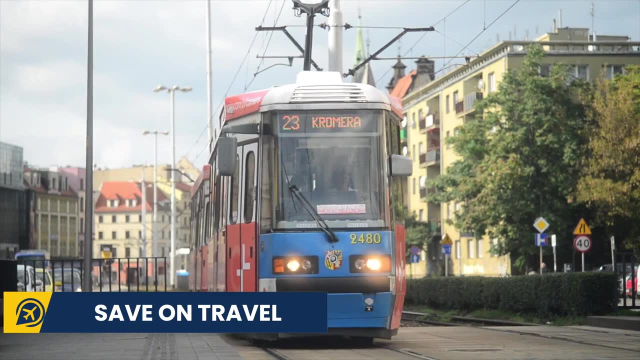 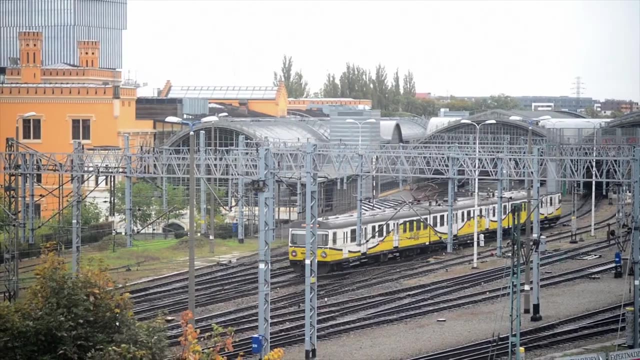 the big chains and opt for the local hotels. You can get some fantastic deals if you look just slightly further away from the city centres. So now let's look at getting around. There are many train routes available in Poland, but they are not as extensive and much more expensive. 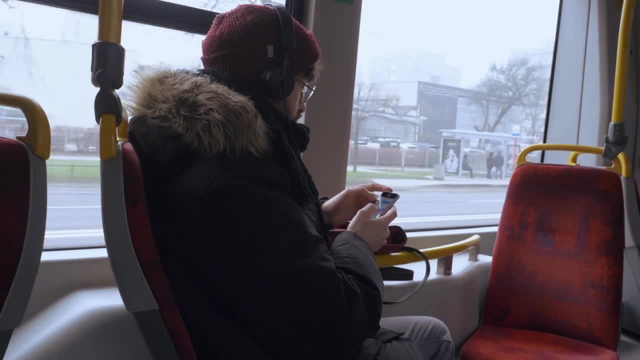 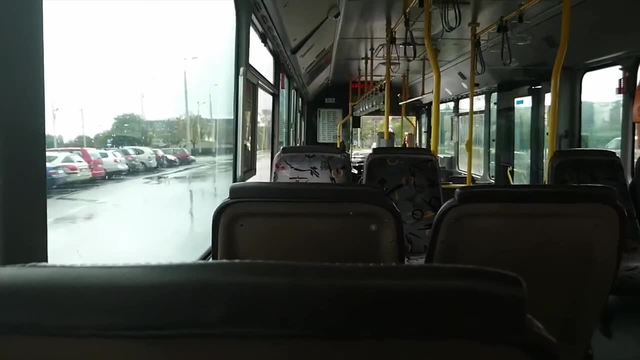 than the bus system. Bus companies have a lot of competition between them, meaning prices are reasonable. Flixbus is the main operator in Poland, so check them out if you are looking to travel across the country. Carpooling is also a popular option in. 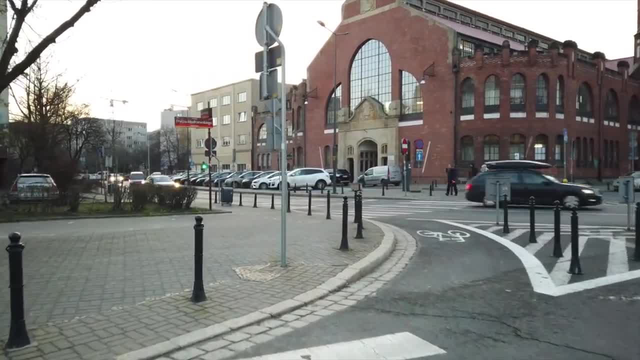 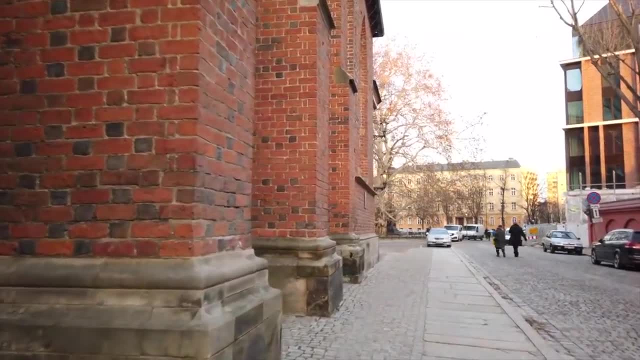 Poland, The website BlaBlaCar has grown in popularity over recent years and can be used to find cheap ride sharing options. All you have to do is search your route and travel dates to share a ride with a local who is driving that same journey. 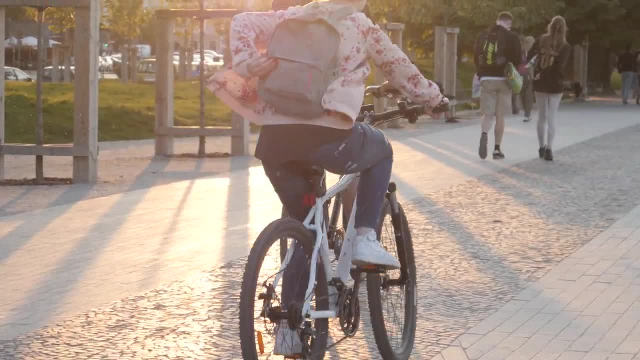 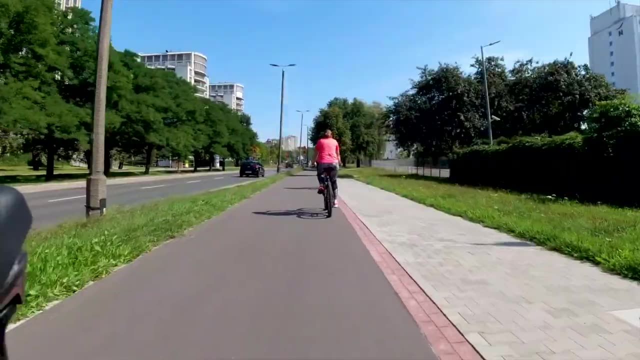 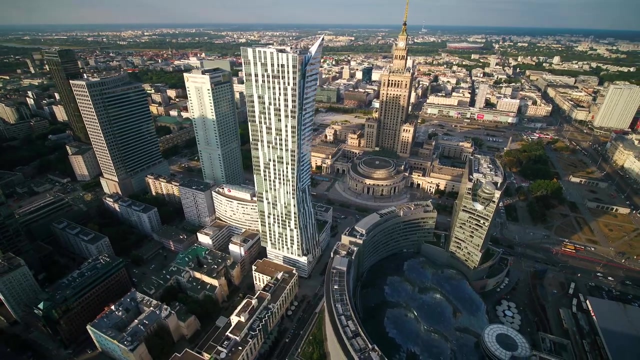 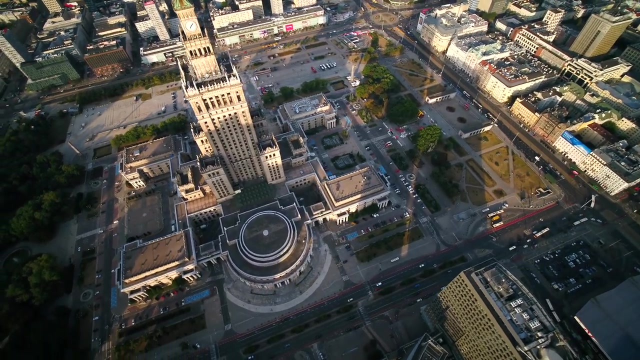 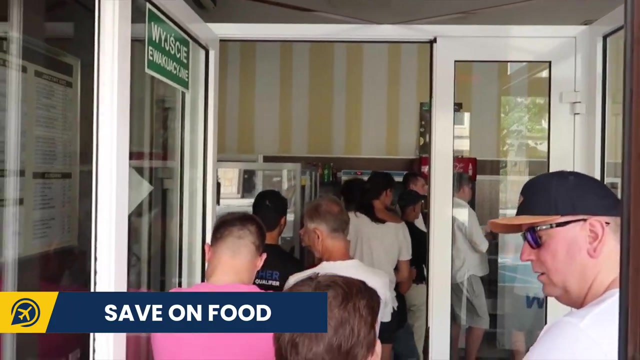 Once you are in the cities, bike sharing apps are also a great way to get around. You can rent a bike for free to ride for around 20 minutes at a time, and there is a small fee for each hour after that. Let's talk about saving money on food and drink. A big way to save money on food and drink in Poland.